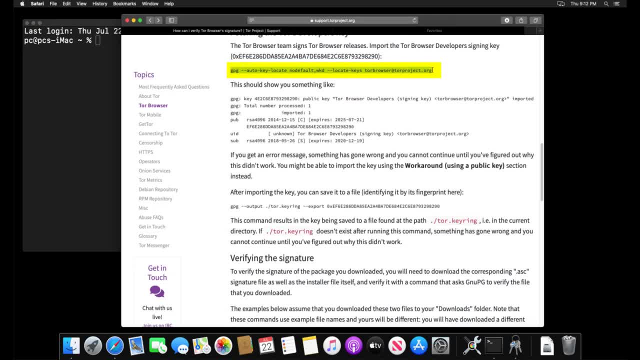 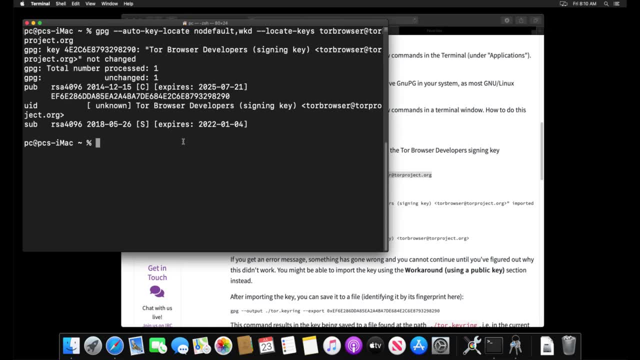 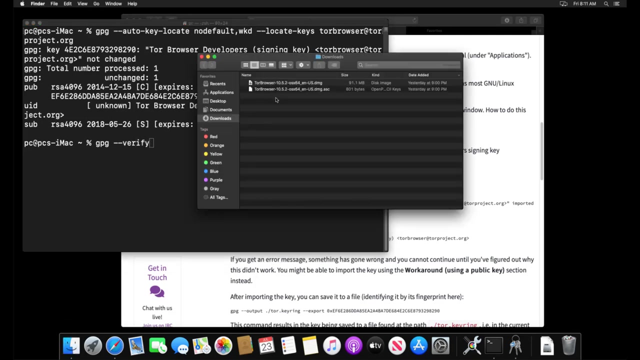 Enter the command to import the developer key. When you enter the command correctly, the developer key is imported, as you can see. After importing the key successfully, let's enter command by specifying the location of the setup file and signature files downloaded. Since the files I download are in the downloads folder, I enter command in this way. 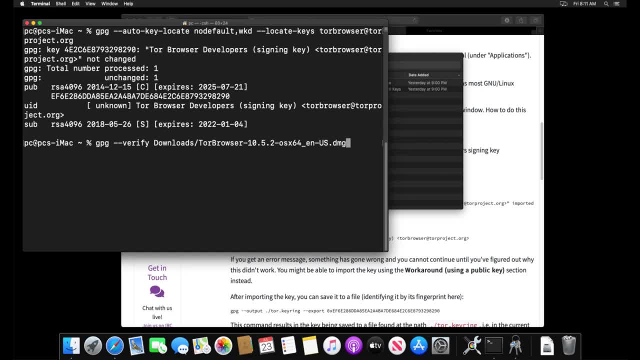 When entering the command, it's important that you first specify the signature file. Let's enter the command. When entering the command, it's important that you first specify the signature file. That is follow the command order. When you click the tab key while typing the file names, the name will be completed automatically. 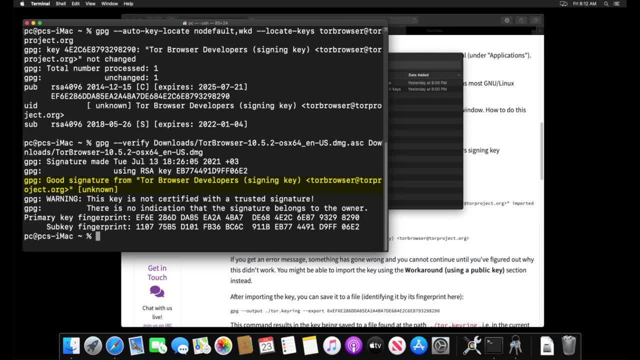 And, as a result, the output I got matched with developer key I imported, proving that my file is signed by the Tor developers and has not been changed or modified. If your file was a modified file, you wouldn't be able to get this output as this signature. 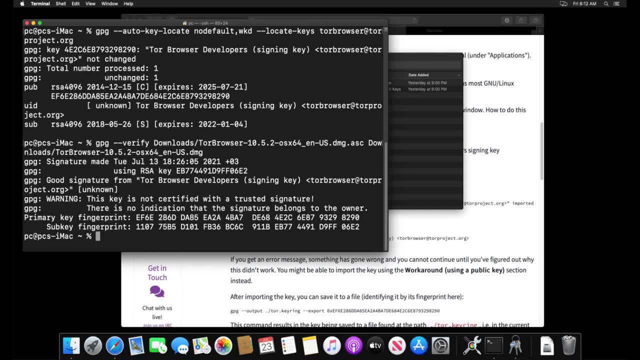 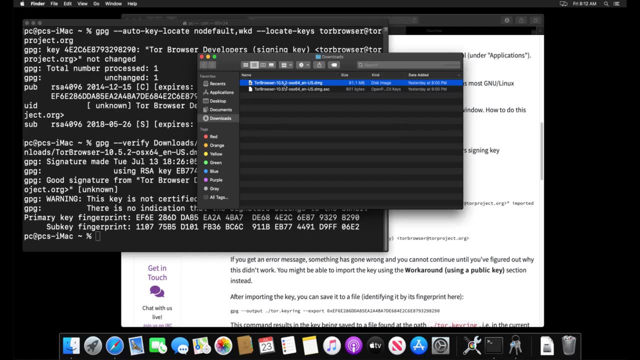 match wouldn't be provided. In this case, you need to download the setup file and verification key from an alternative download source again and try this verification process again. Now that you have verified your file, you can start the Tor browser installation by double clicking the setup file. 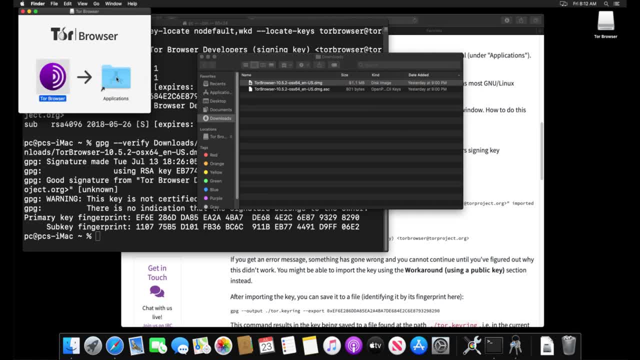 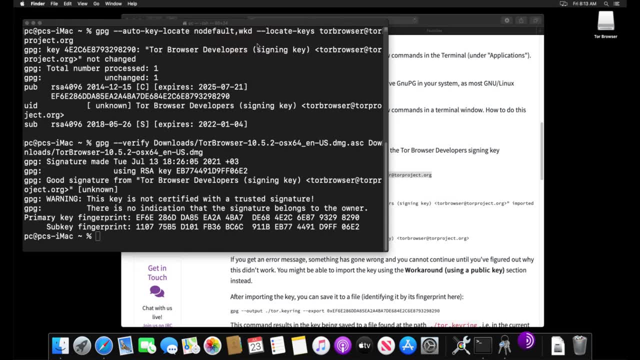 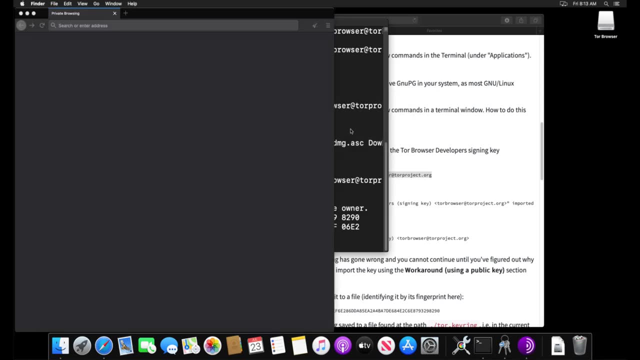 You can drag and drop the application icon onto the application icon to install the Tor browser on your computer. You can run it smoothly. You can run it smoothly. You can run it smoothly by clicking the Tor Browser icon from the application section. In the window that open, you should click the Connect button to connect the Tor Browser. 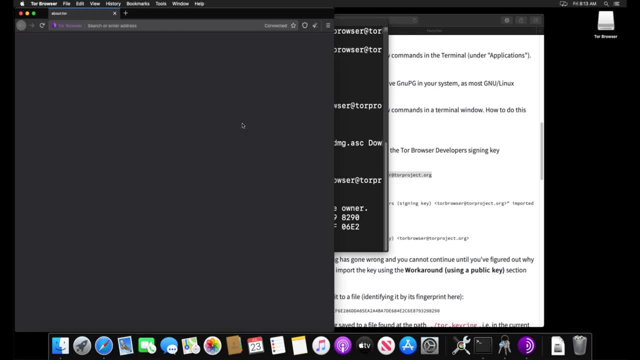 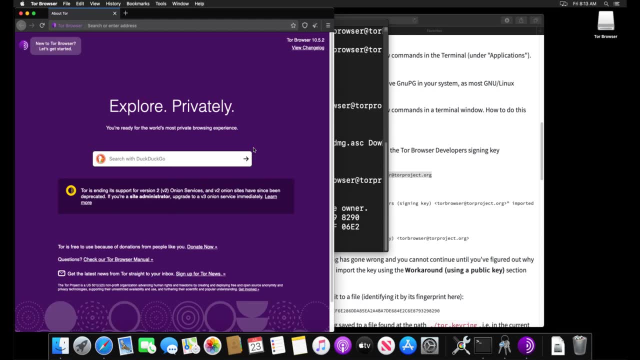 to the Tor network. After a short while, the connection is ready and Tor Browser is opened without any problems. Thus, you have installed the Tor Browser very easily. We will be talking about its use in detail in the following lectures. Finally, I would like to point out that it does not have to perform the verification.